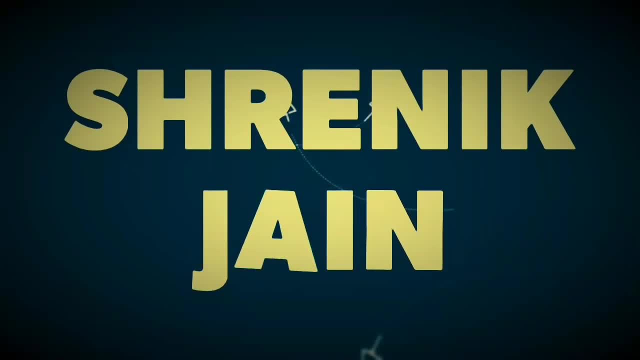 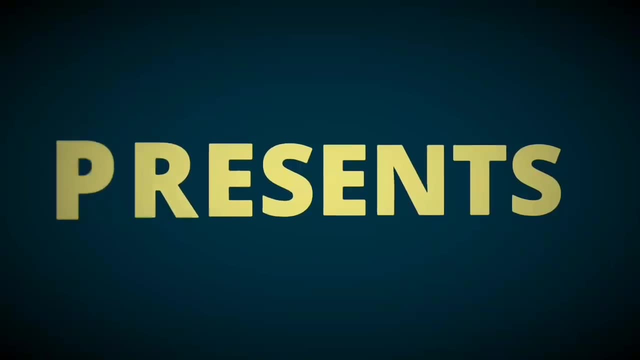 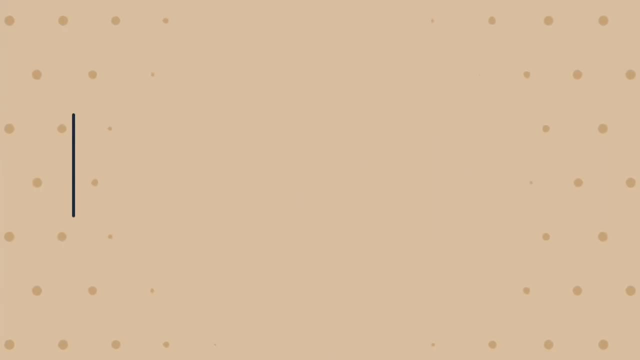 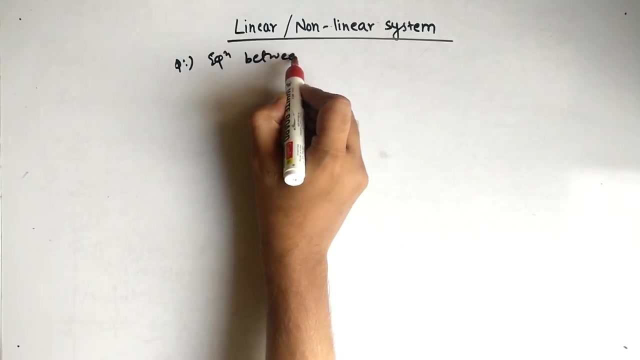 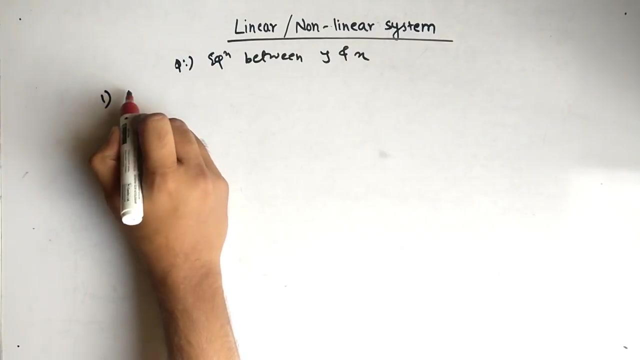 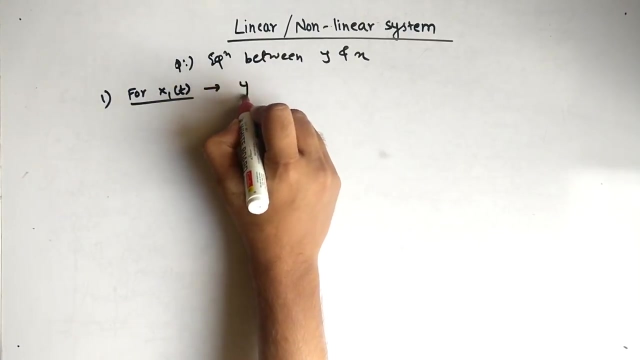 Hello friends, today our topic is how to determine whether a system is a linear or a non-linear system. So we have a question, and the question is equation between y and x. So first step we have to do is find for x1 of t as input, what is y1 of t as output. Similarly for x2. 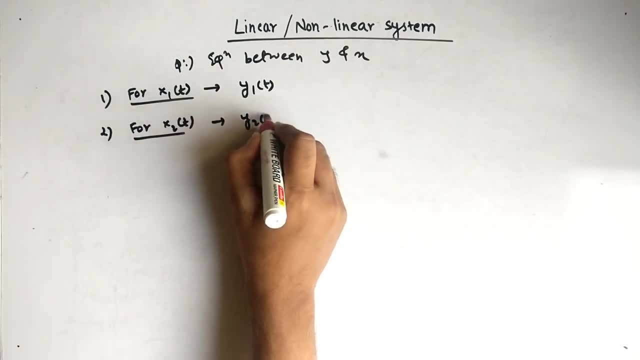 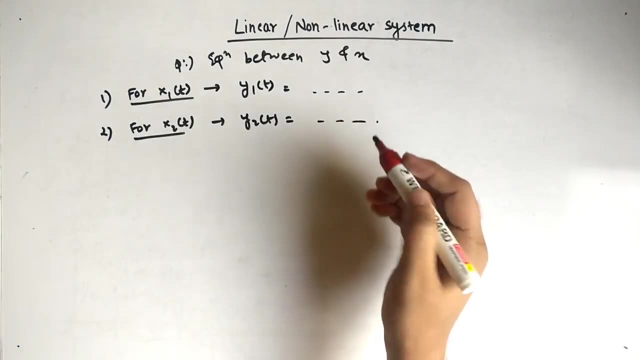 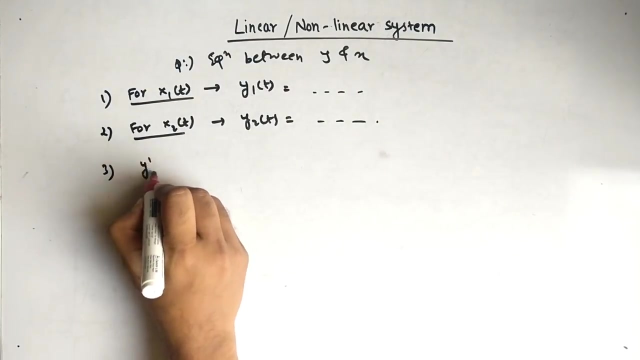 of t as input. what is y2 of t as output? Because there is an equation between y and x. there would be answer over here in terms of x1 of t and here in terms of x2 of t. So the third step we have to do is find y dash of t. So now, what is y dash of t? y dash of. 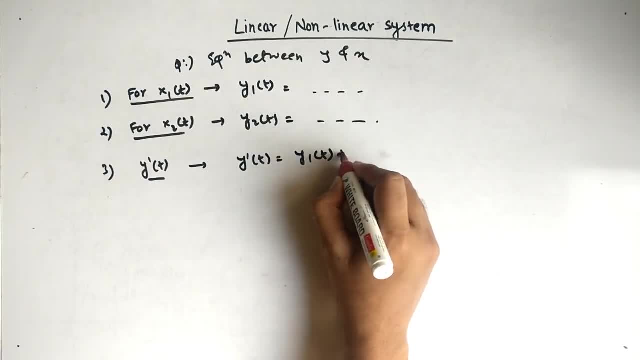 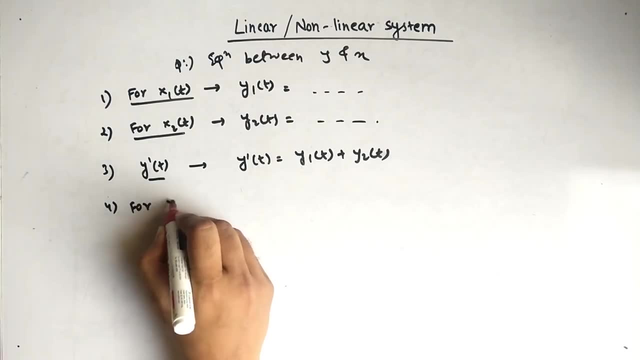 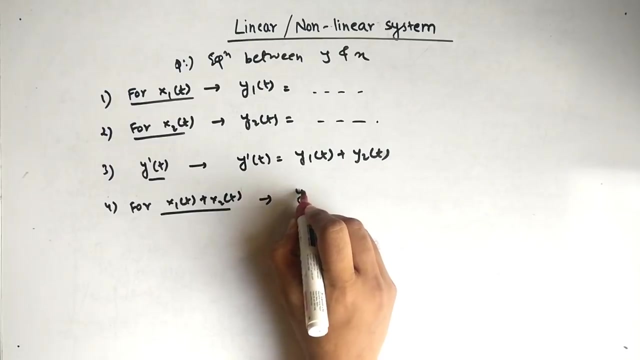 t is equal to y1 of t plus y2 of t. Now the fourth point: For x1 of t plus x2 of t as input, what is the output? And the output is denoted as y double dash of t. Now the last step is to check whether y dash of t is equal to y double. 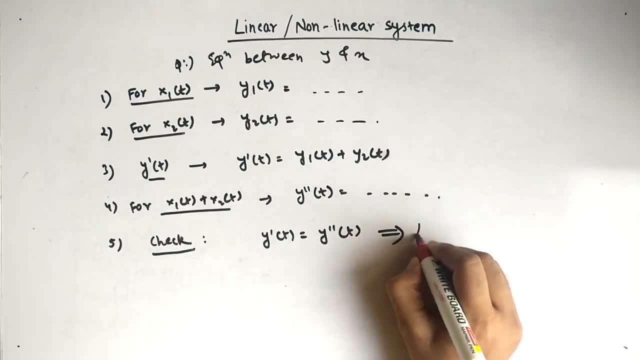 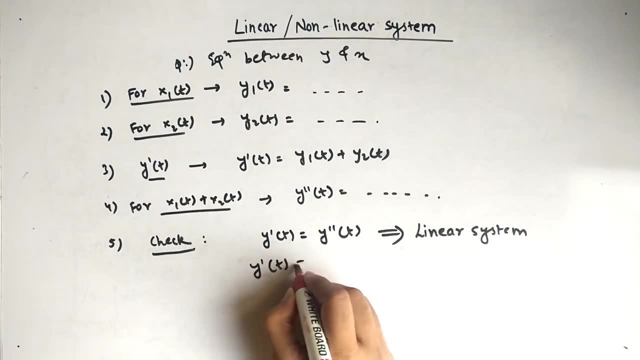 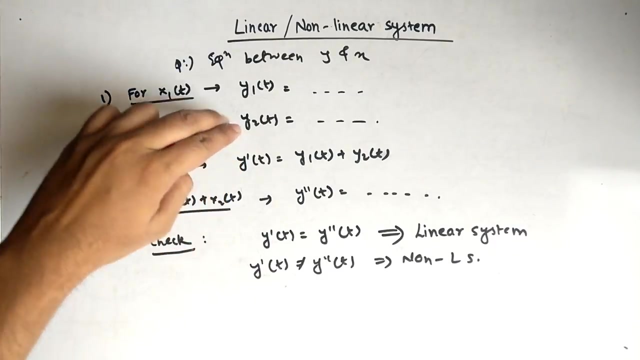 dash of t. If it is equal, then it is linear system. If it is not equal, then it is non-linear system. Okay, So let's take a recap. For x1 of t, what is y1 of t? For x2 of t, what is y2 of t? Then we have to add both: this y1. 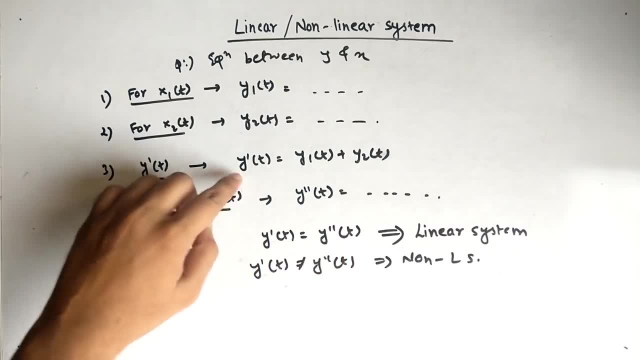 of t plus y2 of t to get y dash of t. Now we have y dash of t. Now we have to find y double dash of t. So for y double dash of t, the input is x1 of t plus y double dash. 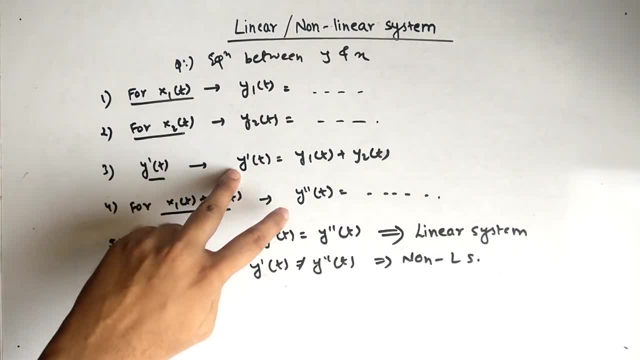 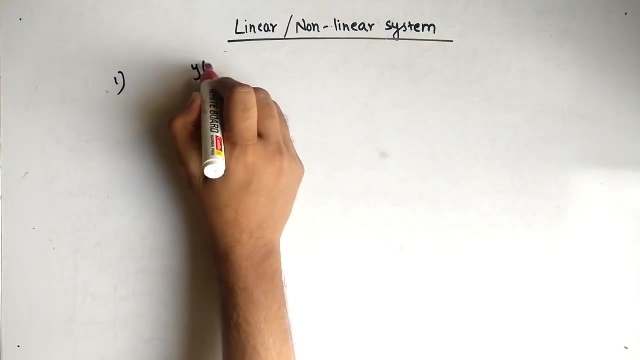 of t plus x2 of t, And then we have to check both y dash of t and y double dash of t. If both are equal, then it is a linear system. If both are not equal, then it is a non-linear system. So let's see an example. So our first example is: y of t is equal to t times x of 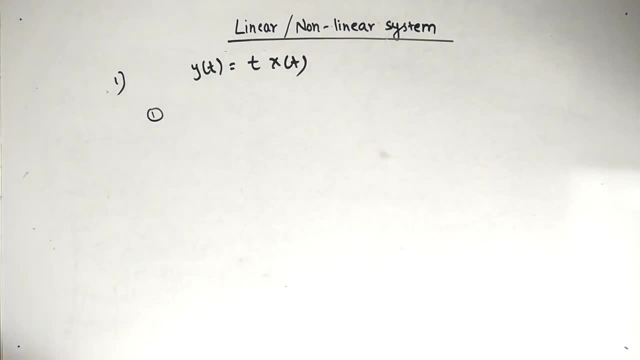 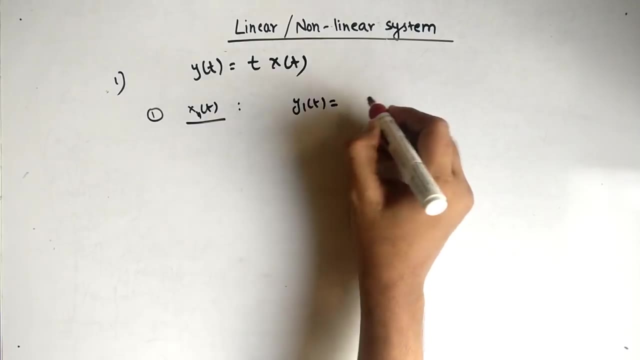 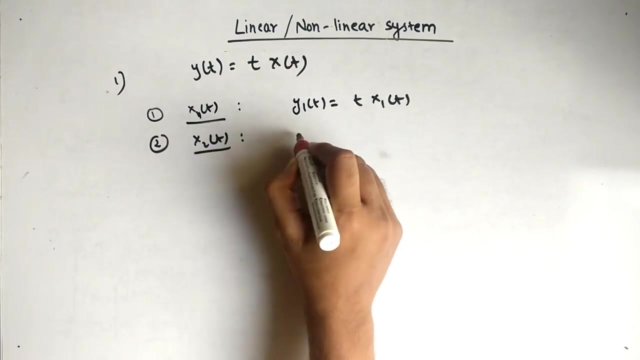 t. Okay. So first step is x1 of t as input. Okay, Then what is the output? y1 of t is t times x1 of t. Okay, Fair enough. Now taking x2 of t as input, Again y2 of t is equal to. 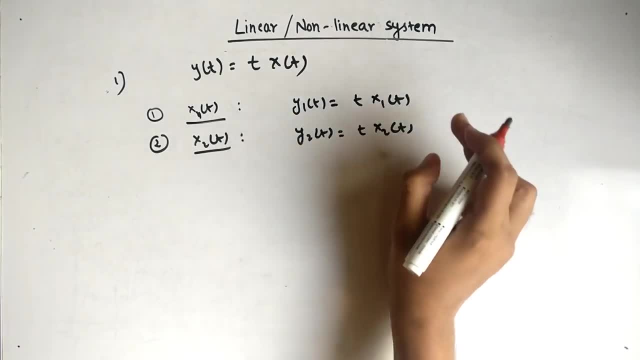 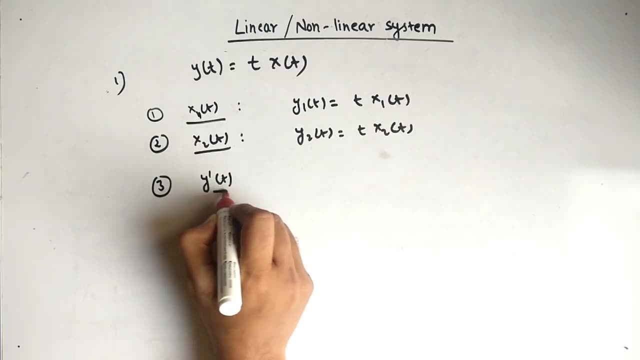 t times x2 of t. This remains same t and only the function x of t changes to x1 of t. Simple. Now third step. Third step is y dash of t. Y dash of t is what Y dash of t is: y1 of. 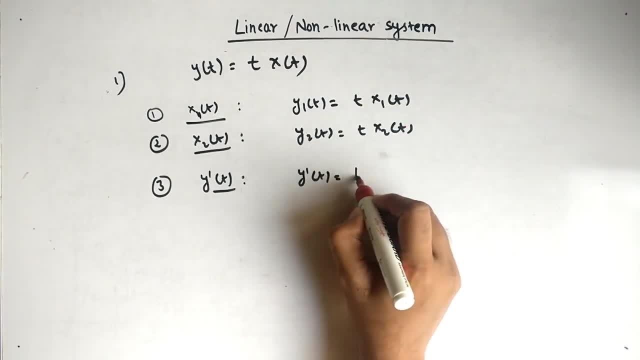 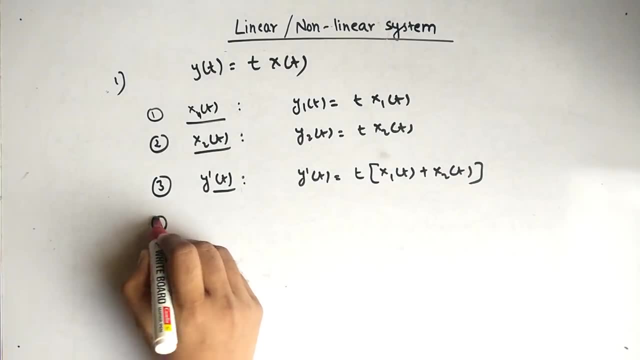 t plus y2 of t. This means adding these two. Okay Now, t is common, So we have to find x1 of t plus x2 of t. Now the fourth step Input is x1 of t plus x2 of t. Okay, These. 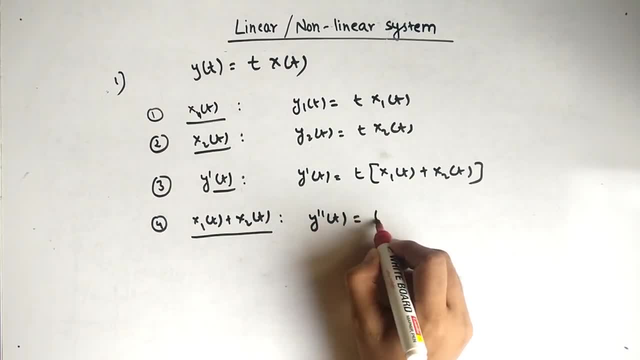 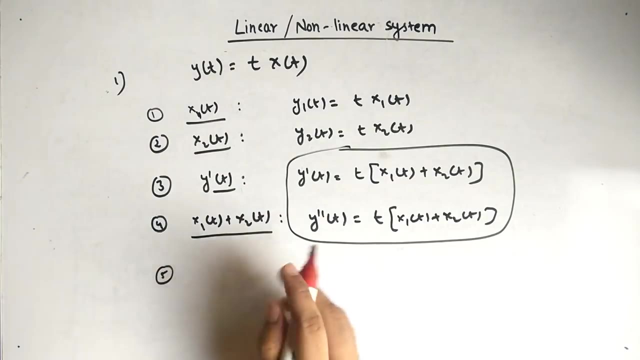 are our inputs. So what is now y double dash of t? t remains as it is Now x of t changes to x1 of t plus x2 of t. Now you can see these. both Are they equal? Let's check. Yes, Both. 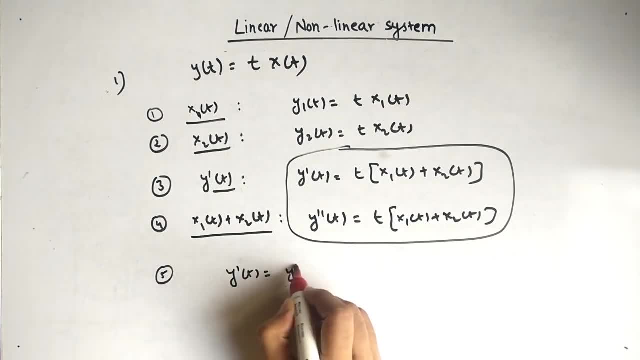 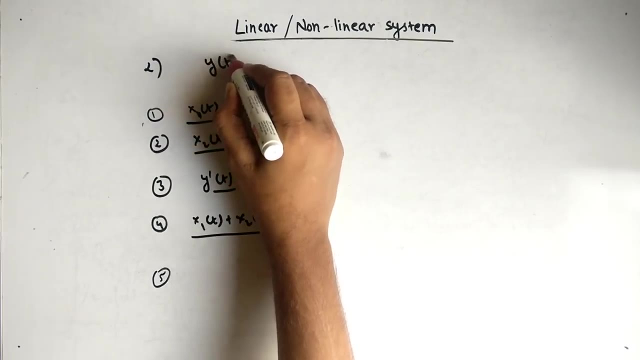 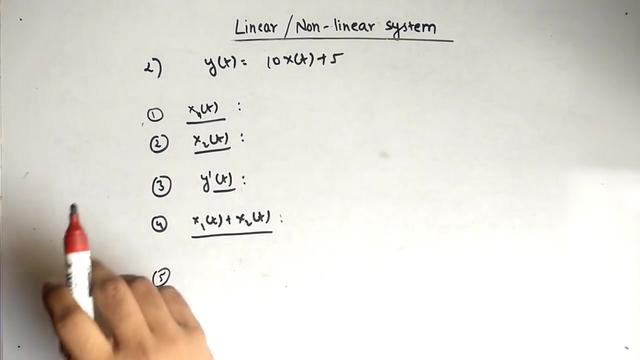 are equal. So y dash of t is equal to y double dash of t. This means system is linear. Now let's take one more example. Now the second question is: y of t is equal to 10 times x of t plus 5.. So what is the first step? x1 of t as input. So y1 of t is our output, and 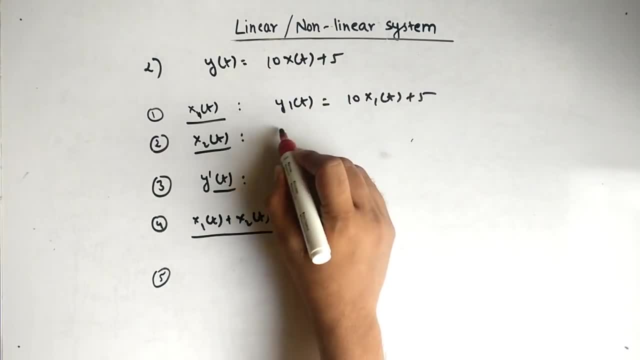 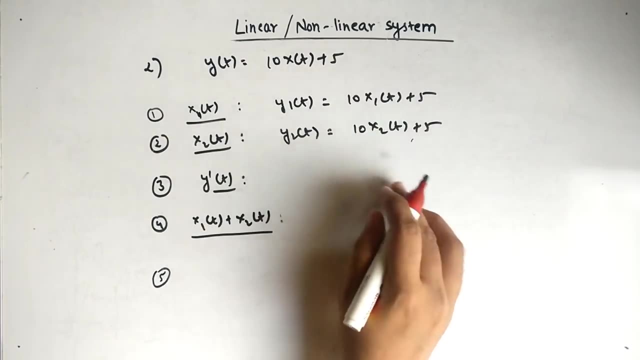 that is equal to 10 times x1 of t plus 5.. Similarly, y2 of t is our output and x2 of t is our input. So 10 times x2 of t plus 5.. Now y dash of t was adding both. If we add, 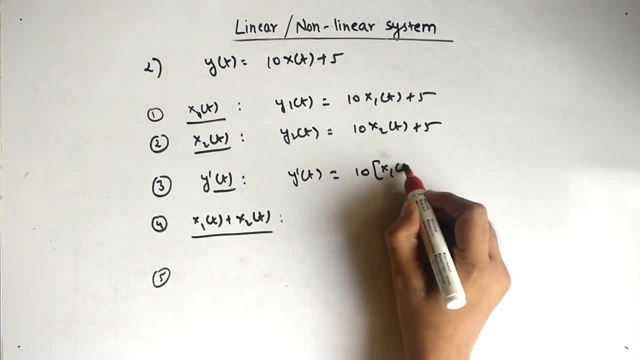 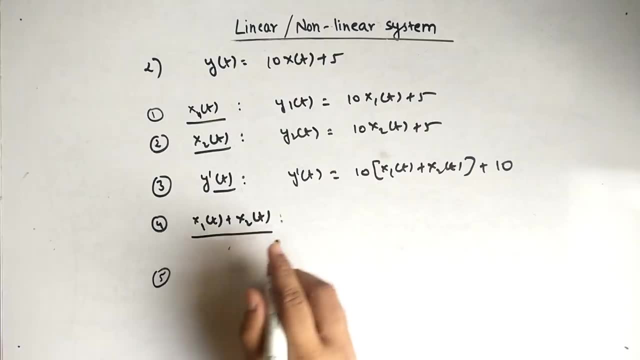 both we get 10 as common and these two inside the bracket. Okay, But these two gets add again, so we get 10 here. Talking about this, the y double dash of t as our output, and in input is this Now changing x of t to x1 of t plus x2 of t, So again 10 as the multiplying. 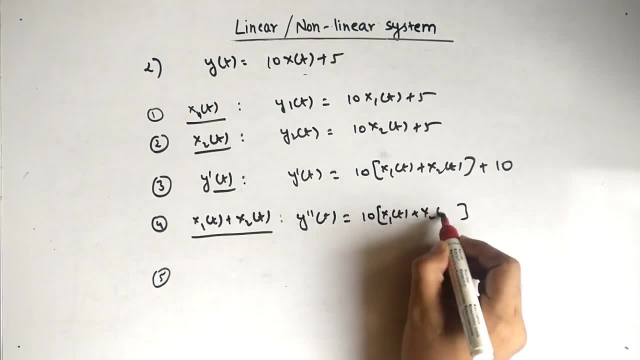 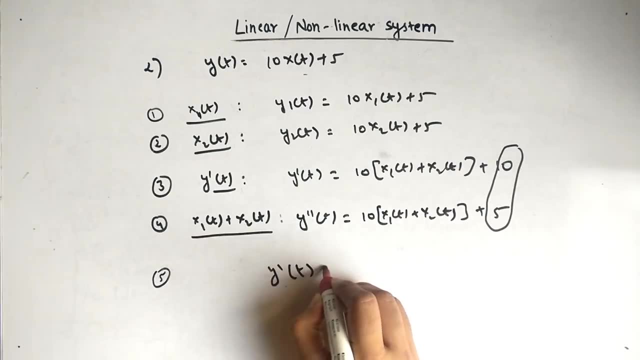 factor and inside the bracket we have x1 of t plus x2 of t, But now we have only plus 5.. So you can see the difference. So y dash of t is not equal to y double dash of t. This means system is non-linear system. Okay, Now let's see some of the example that comes under. 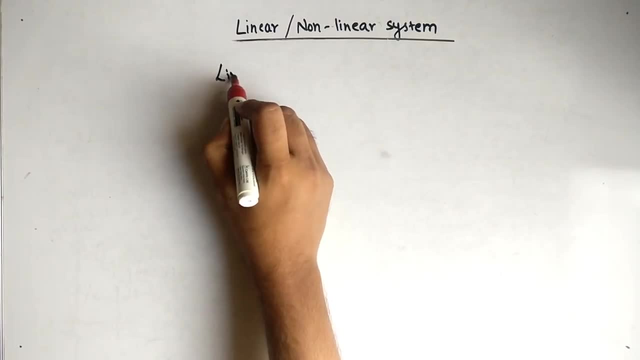 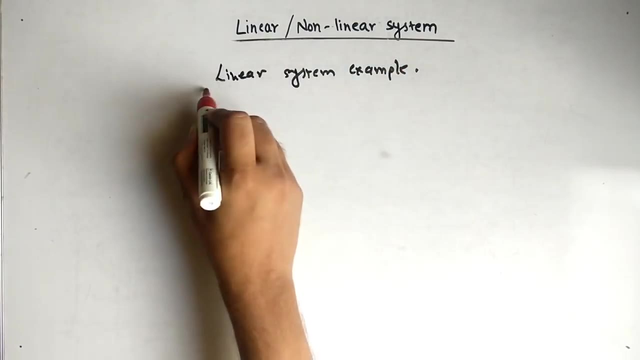 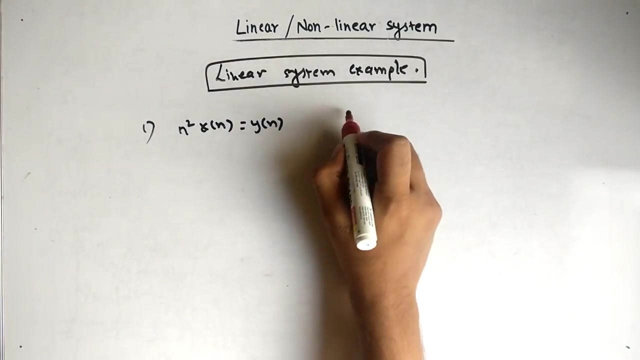 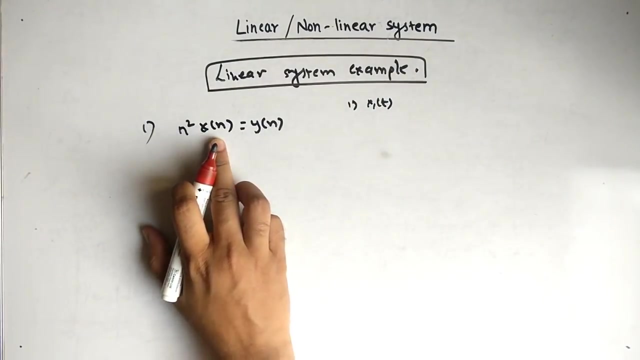 linear system. So linear system example. So first example is n square x of n, That is equal to y of n. Now let's orally solve this. So first we have x1 of t as input. t was for the continuous time. So if we change t to n, then we get discrete time. Alright, So now. 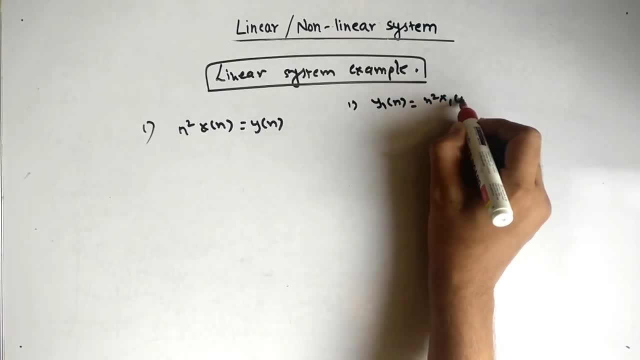 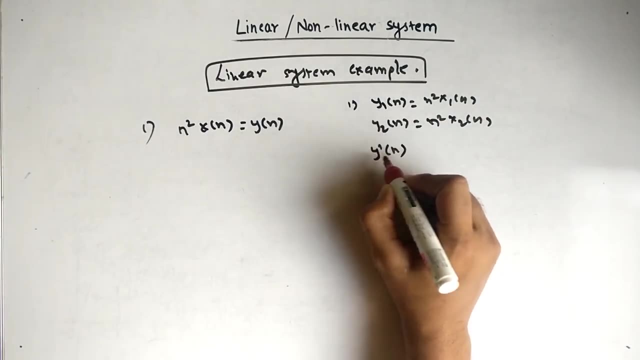 we have y of y1 of n, That is equal to n square x1 of n. Alright. Then we have y2 of n, That is equal to n square x2 of n. Then we add both this, So we get y dash of n. Adding these: 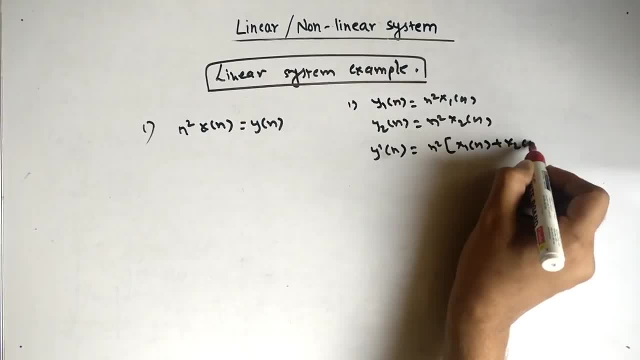 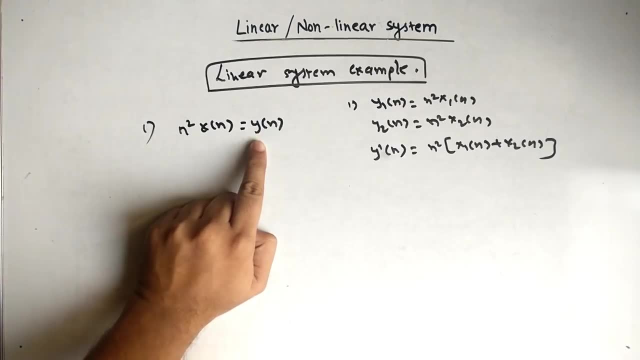 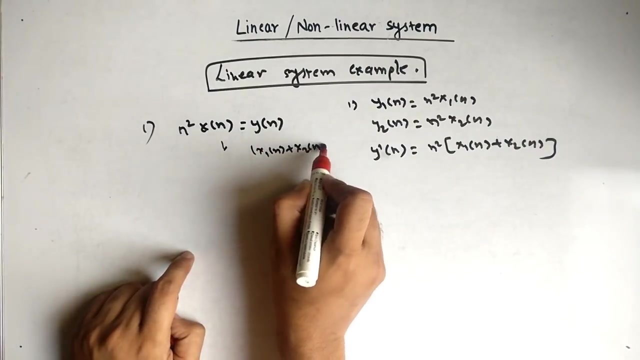 two, we will get x1 of n plus x2 of n. Alright, Now just imagine that we are finding y double dash of n. Y double dash of n means changing x of n to. We change this to x1 of n plus x2 of n. Alright, 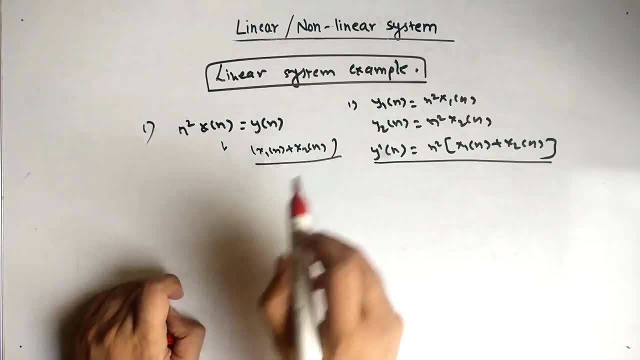 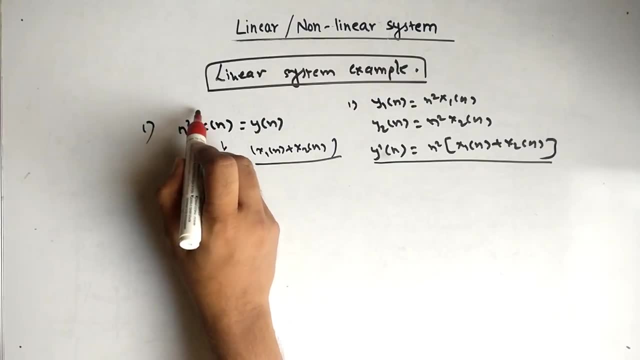 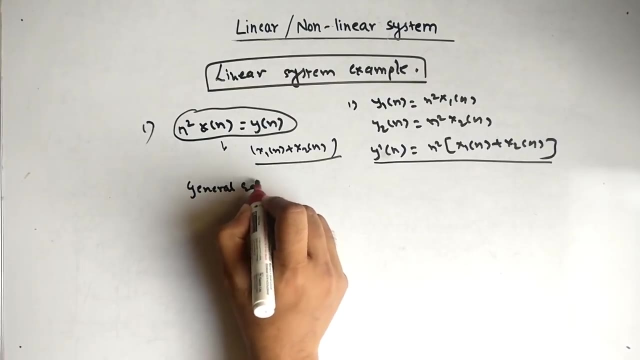 And changing this, we will get the same answer. So you can see both are equal: Y dash of t and y double dash of t. This means it is a linear system. So what this mean. This equation gives a very general equation. Alright, So the general equation is that if we have y, 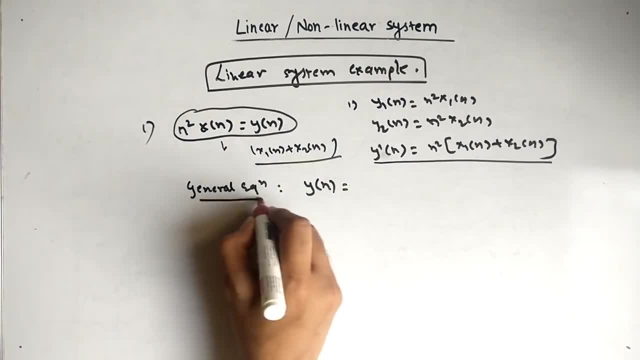 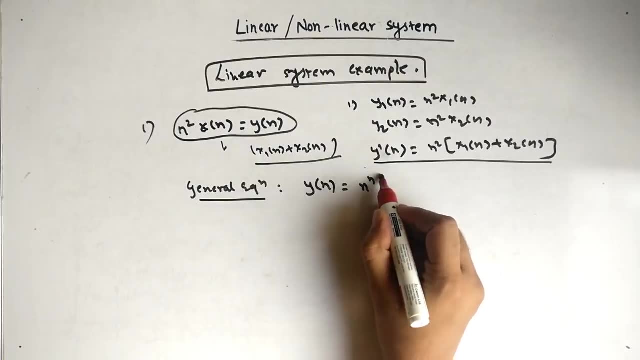 of, let's say t or n. I'm taking n here. Alright, The general equation is: y of n is equal to t. Let's say n is the variable. So n raise to n. Again, n can be any value, 1,, 2,, 3,, 4, any value. And we have 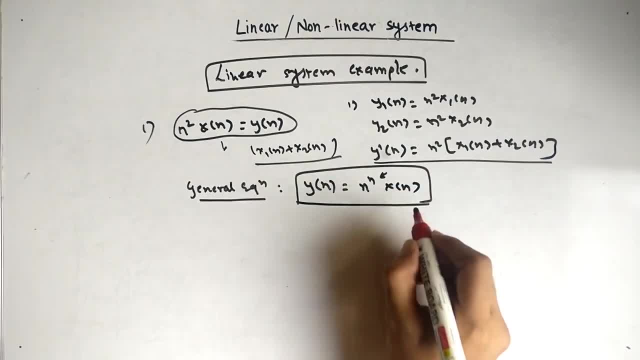 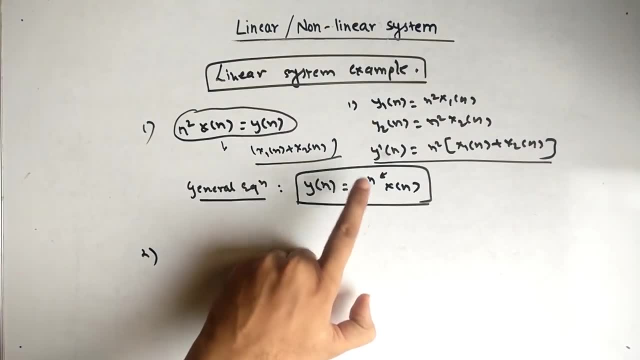 x of n. If you see this, This equation, This means it is a linear equation. Alright, This was multiplying n raise to n, Alright, And this small n means any value: 1,, 2,, 3,, 4, anything. 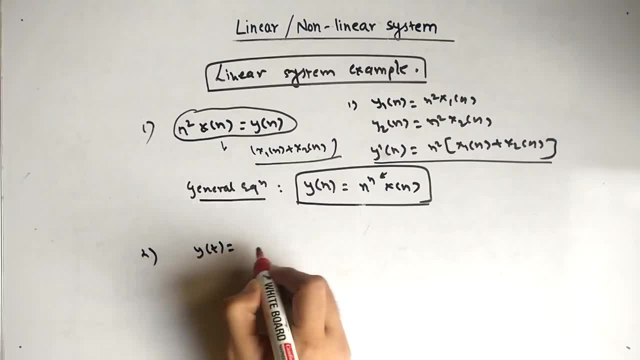 What if y of, let's say t, is equal to t? Alright, So this is a linear equation. Alright, So x of n is equal to 10 times cos of, let's say 100 pi t And multiply by x of n. Sorry, 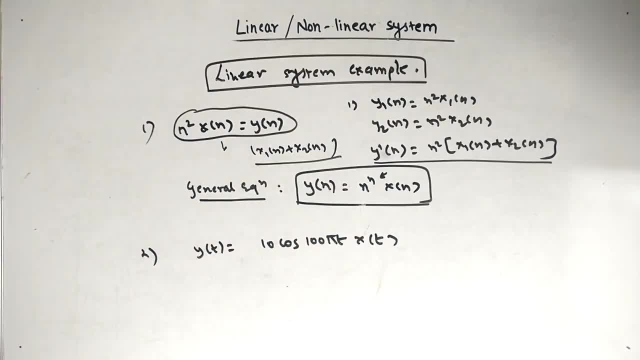 t is the variable, So x of t. What will be the answer for this? Now again, you multiply this and you got it is a linear system. Now, when you change this, also Like x1 of t and x2 of t, What changes? is this Alright? Then we will get this Alright. So x of n is equal. 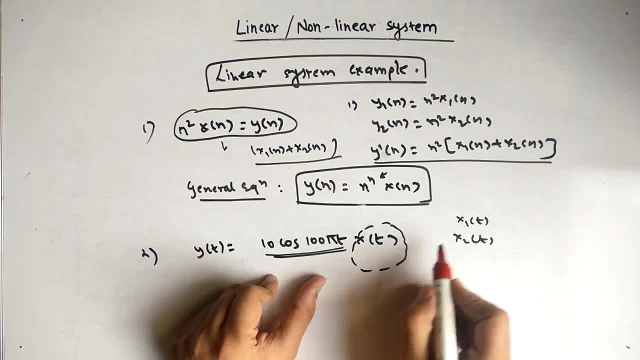 to 10 times cos of, let's say, 100 pi t. And when you change this also, Like x1 of t and every variable are the same, Alright, This remains same in both. Alright, So 10 times cos of, let's say, 100 pi t Remain same In both. Now variable changes. So when we add 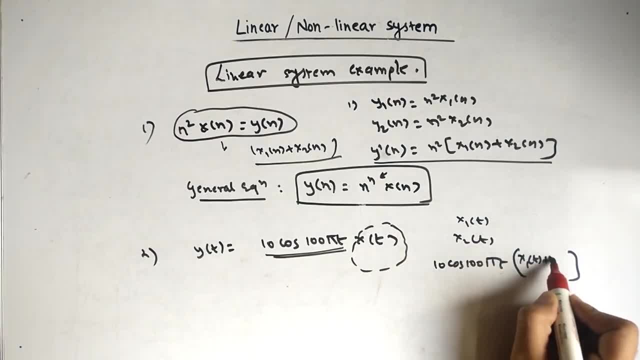 only these two variable adds Alright, and we get y dash of t. Fair enough, Alright. Let's say one more time: x1 of t will be 10 times cos of. let's say 100 pi t with x1 of t, and x2 of t will be 10 times cos of. let's say 100 pi t, x2 of t with x2 of t. Then we 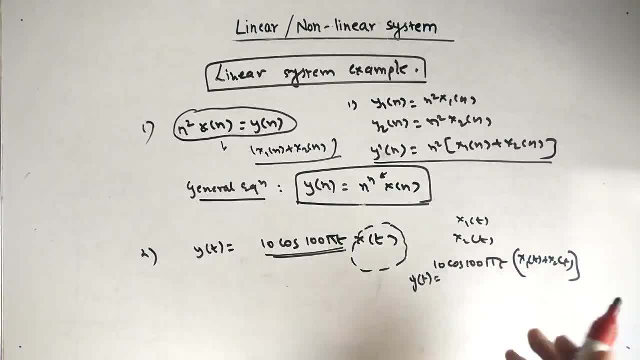 we add, then we get this and we get y dash of t. now talking about y double dash of t, what will happen? only this will change. and this will change to x1 of t plus x2 of t. so again both are equal. y dash of t is equal to y double dash of t. this means the system is linear system, so this can be. 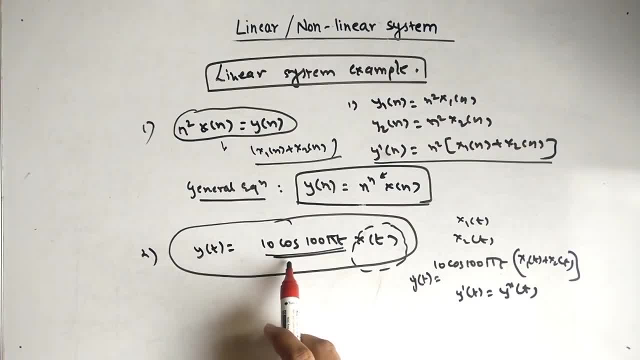 also a general equation, all right. when we multiply anything, anything to x of t, we get a linear system. now the important point here is: suppose i add, suppose i add. let's say anything, either n, square, or let's say 10 cos, pi, t, if i add any constant to them. let's take example t, q and it. 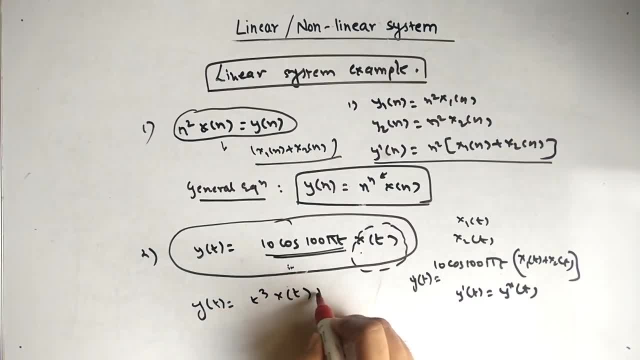 is x of t. i have this, and now i add a plus 10. what will happen? what will happen is: x1 of t. we get a plus 10 here, all right, you. and in x2 of t, we also get all right, this will happen. we are solving this t cube, x1 of t plus. 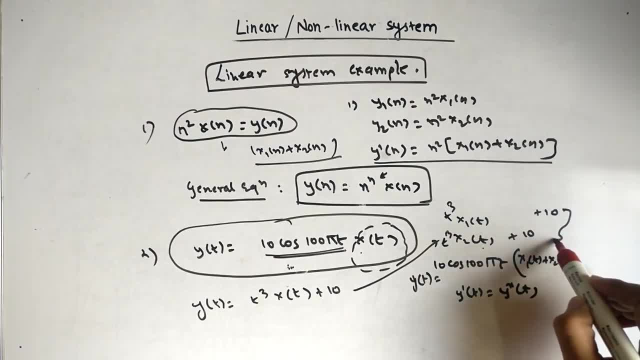 10 t cube x2 of t plus 10. now when we add both this 10 plus 10 also added, and we give and we get 20 and 20 is in y dash of t. but when we solve for y double dash of t, what will happen? 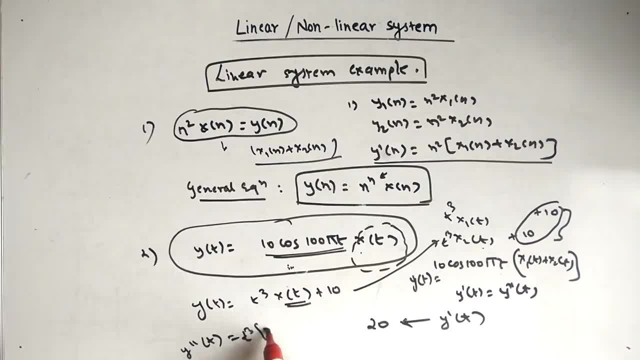 only this changes. this changes to t cube here x1 of t plus x2 of t and 10 remains at as it is. this is not 20 here, so 10 as it is. so what is difference? the constant changes all right. when the constant changes both, the equation changes y dash of t, y double dash of t. this 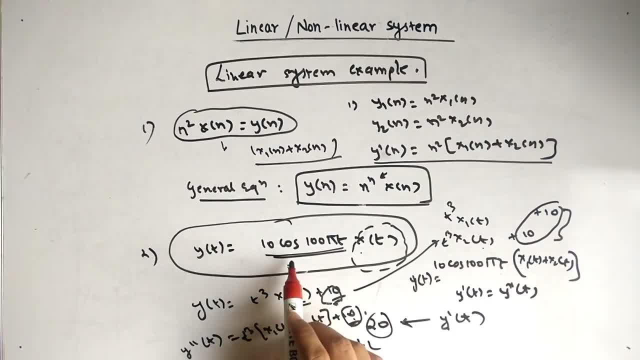 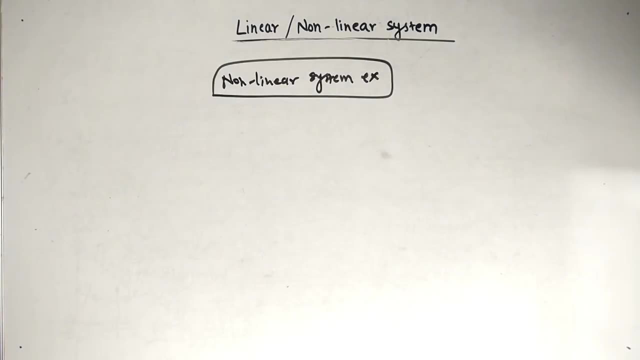 mean is non linear system. so remember this, this: this are linear system. but when we add a constant, u see, when we add a plus c, when we add a plus c, it becomes a non linear system. now let's see the example of nonlinear system. so first we had is we talked previously, that is, if we have 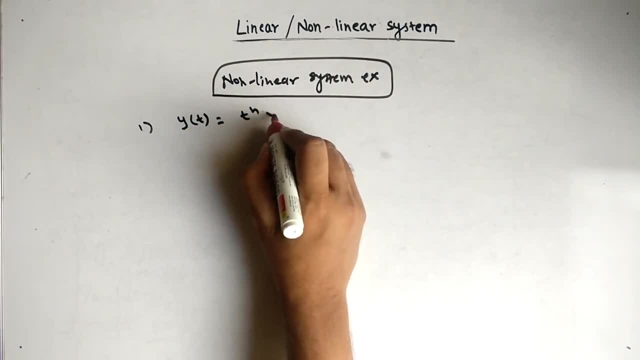 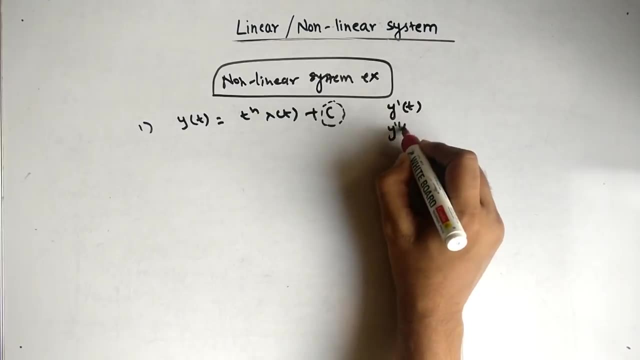 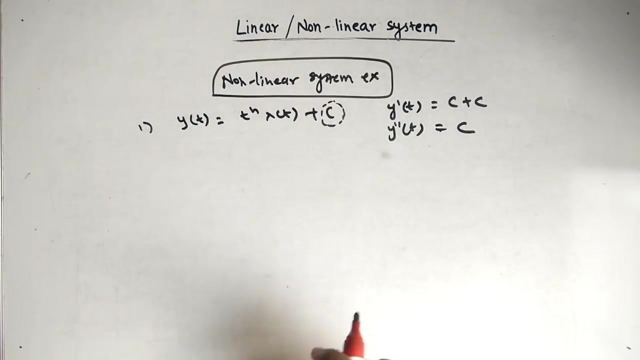 y of t and let's say t raise to n x of t and we add a constant. this constant changes for y dash of t and y double dash of t. what happens is we get constant added right here, but here we have only one constant, so these two are not equal. this means it is a nonlinear system. when we talk about second, 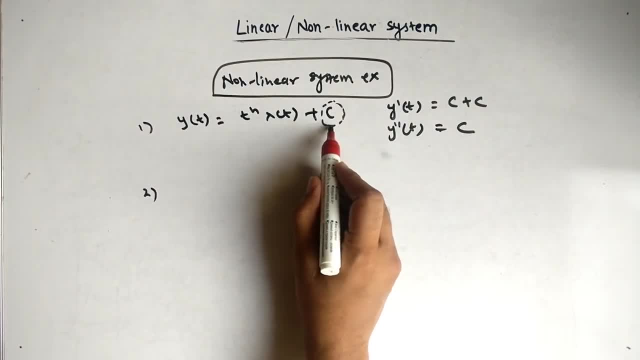 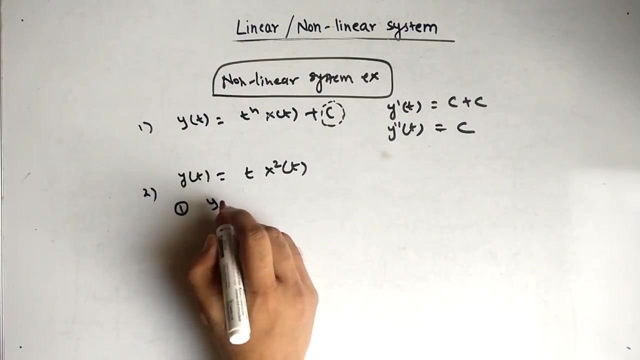 example. the second example is here. we added constant in this. what about we square this? so if we have y of t that is equal to, let's say, t into x, square of t, now what will happen? let's solve this. so first step is finding y dash of t. all right, for this we need two y, one of t and y. 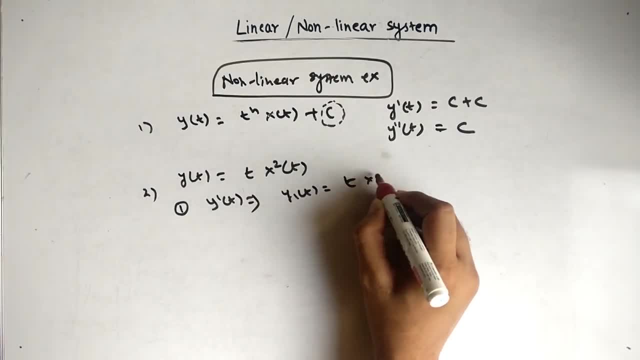 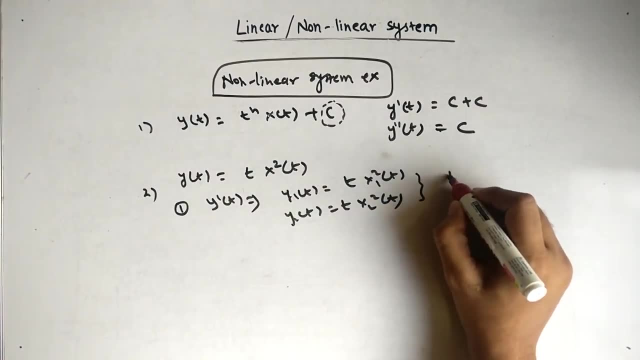 y two of t. so y one of t is t times x one square of t, and y two of t is t times x two square of t. all right now, adding this two, we get t common, but x one of square, this to get added, so x one square. 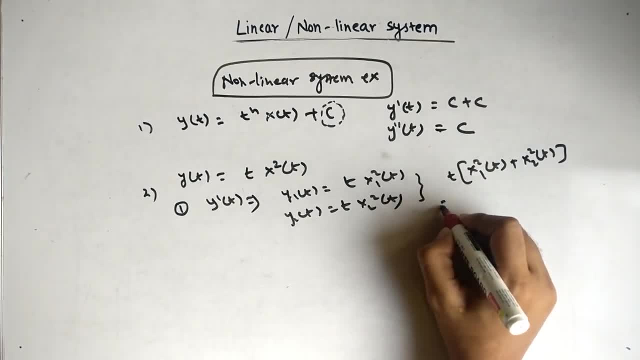 of t plus x two square of t. so this is nothing but y dash of t. all right, now we have y dash of t finding y double dash of t. for y double dash of t we need x of t. change to x. one of t plus x two of. 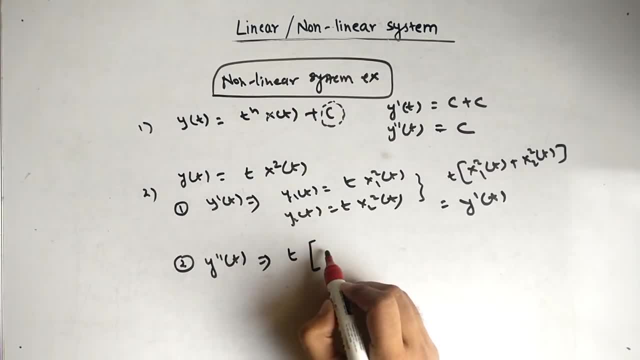 t. so what will happen right here? this is important. see: x one plus x two. all right, let me write this way: x one of t plus x two of t, and it will become the whole square. all right, now you can see. now you can see the difference. so this is the whole square. why see closely? we have x. 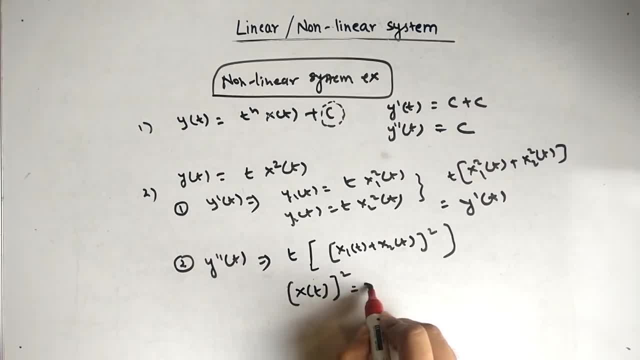 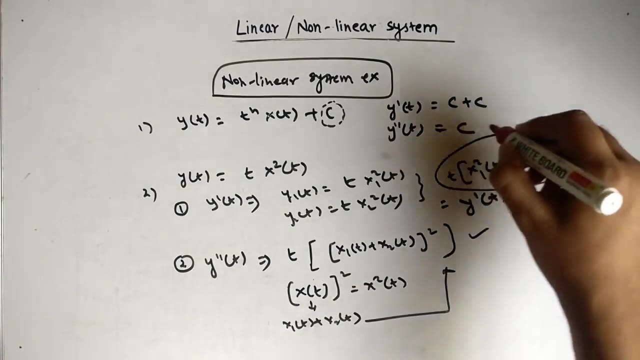 of t, the whole square. this means this: and this are equal: x- square of t. all right, now we are replacing x of t to x 1 of t plus x 2 of t. that's why we get this all right, and you can see this: and this are not equal. 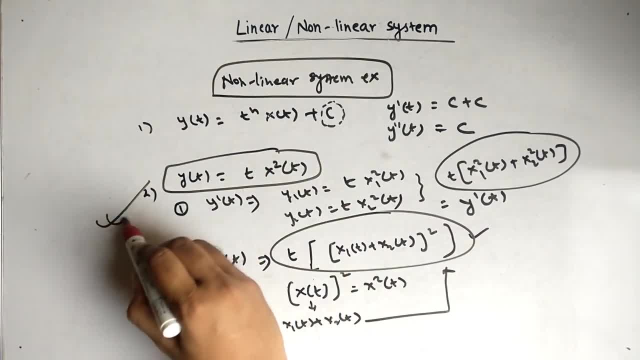 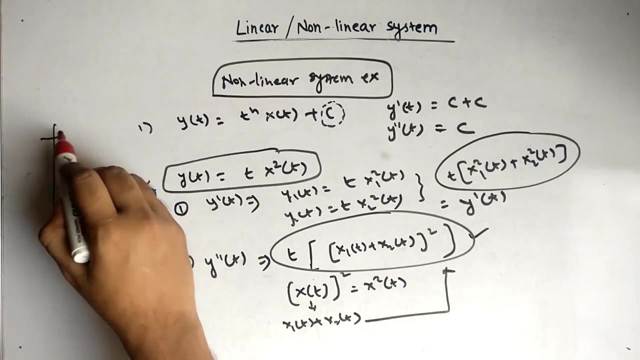 so again, this equation is very important. so this gets added to a non-linear system. what if i had x of t square and not x square of t? then this is linear, now y it is linear solid. when you solve it, we get x 1 of t square. 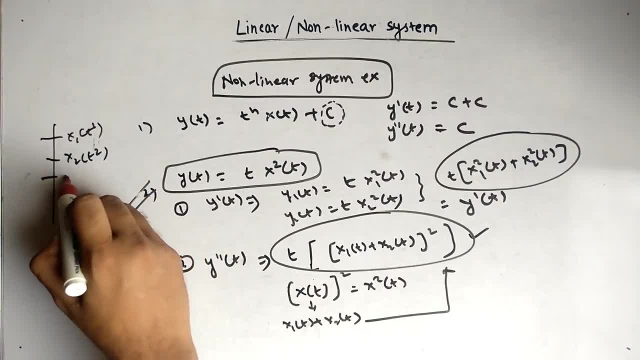 x 1 of t square, then we get x 2 of t square. then we add: then we get x 1 of t square plus x 2 of t square. now, when we change this- now let's see closely- we have this. all right, we are changing. 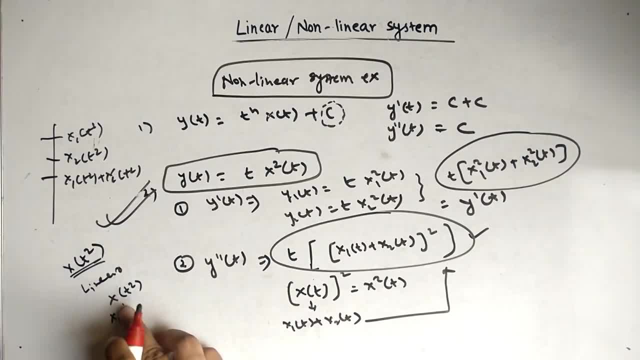 only this x 1 of something. let's say, right, this way: x 1 of something plus x 2 of something. this and this will remain same. so y dash of t and y double dash of t remains same. but here, when we replace x of t, we get x1 of t plus x2 of t. the whole square. you can see the whole square. 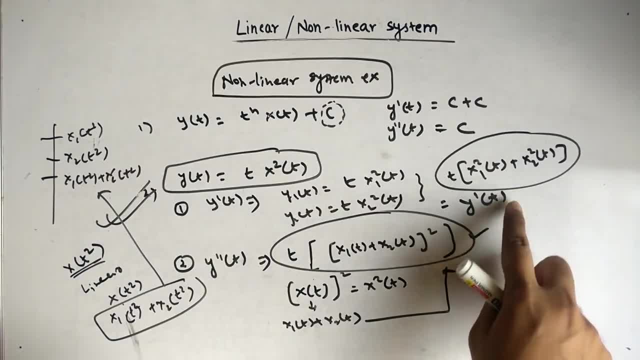 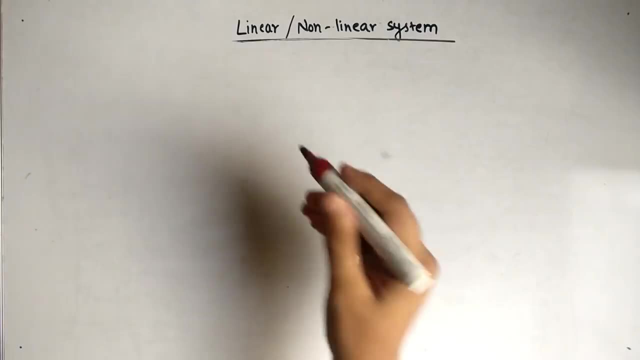 and here the equation equation is different. that's why this is very important example and don't get, don't get confused between x square of t and x of t square. now let's take the last, very important equation, and the equation is: y of t is equal to e raised. 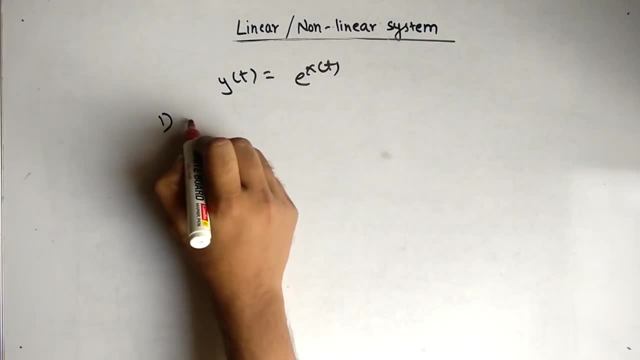 to x of t. let's solve this: first: x1 of t as input, then we get y1 of t, that is equal to e raised to x1 of t. all right. then we have x2 of t, and y2 of t is equal to e raised to x2 of t. all right now.